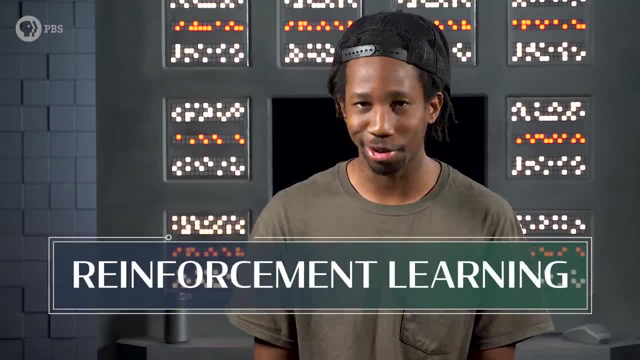 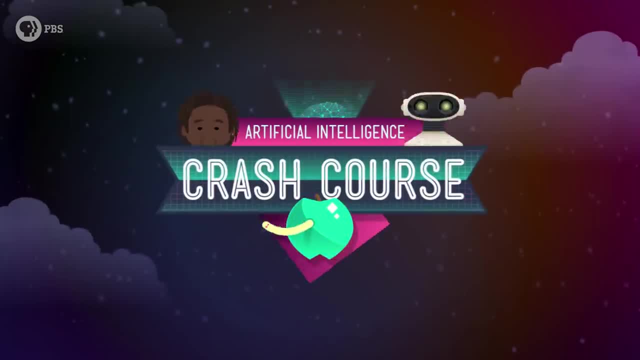 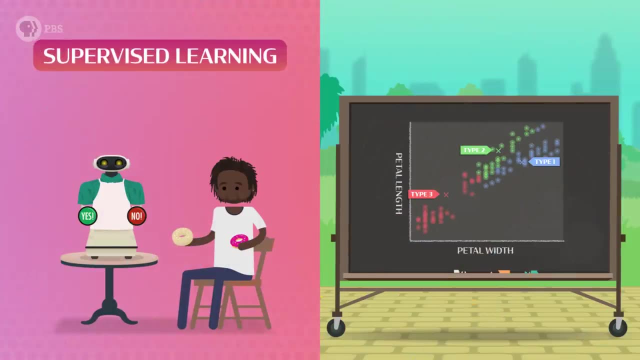 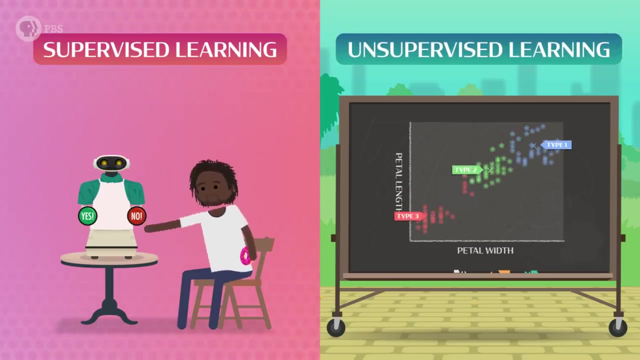 complicated goals is called reinforcement learning. So far we've talked about two types of learning in Crash Course: AI: Supervised learning, where a teacher gives an AI answers to learn from, and unsupervised learning, where an AI tries to find patterns in the world. 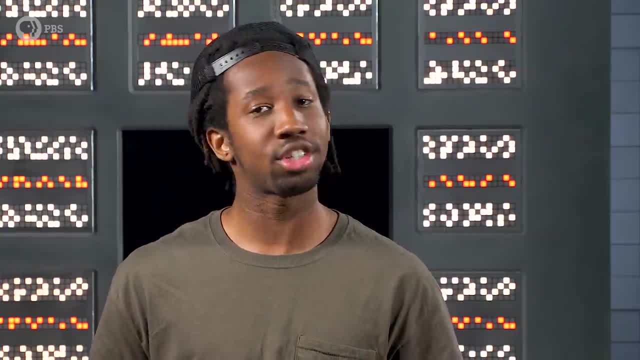 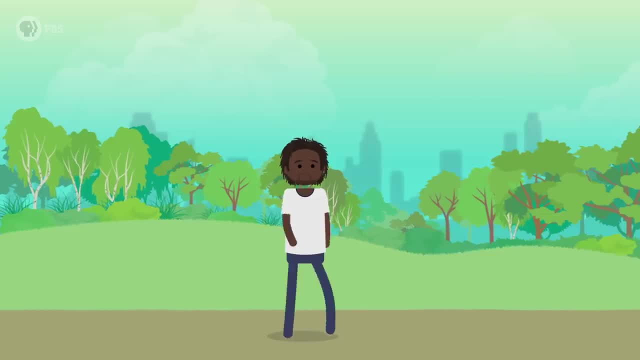 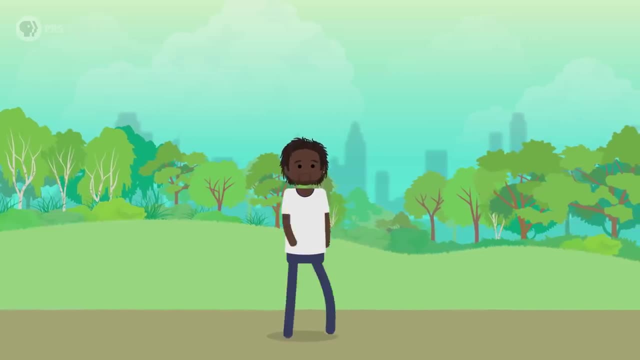 Reinforcement learning is particularly useful for situations where we want to train AIs to have certain skills we don't fully understand ourselves. For example, I'm pretty good at walking, but trying to explain the process of walking is kind of difficult. What angle should your femur be relative to your foot And should 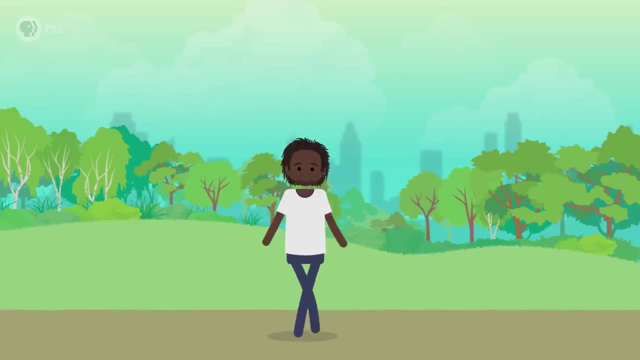 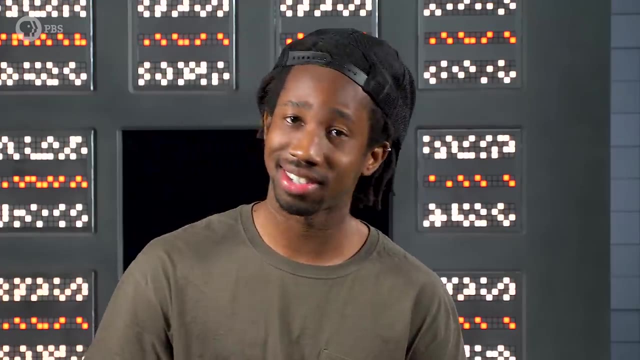 you move it with the average angular velocity ofyeah, never mind, It's really difficult. With reinforcement learning, we can train AIs to perform complicated tasks, But what's more, unlike other techniques, we only have to tell them at the very end of the task if 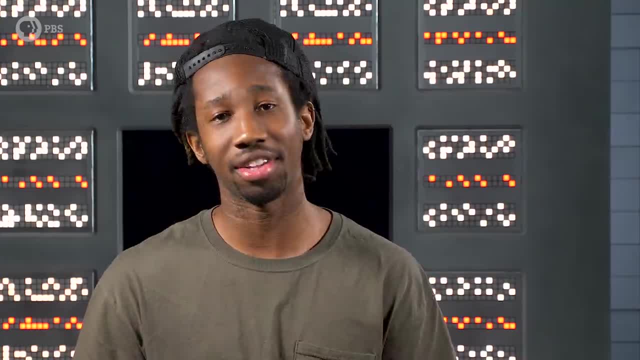 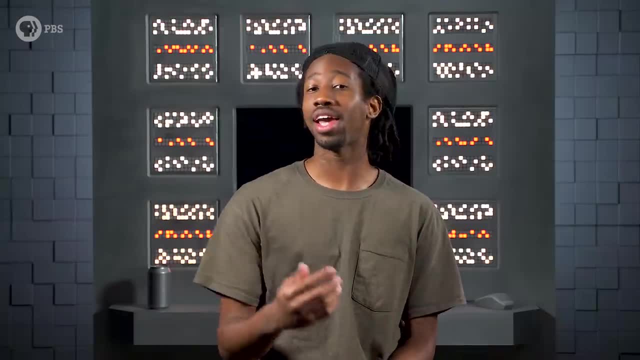 they succeeded and then ask them to tell us how well they did. We're going to focus on this general case, but sometimes this feedback could come earlier. So if we want an AI to learn to walk, we give them a reward if they're both standing. 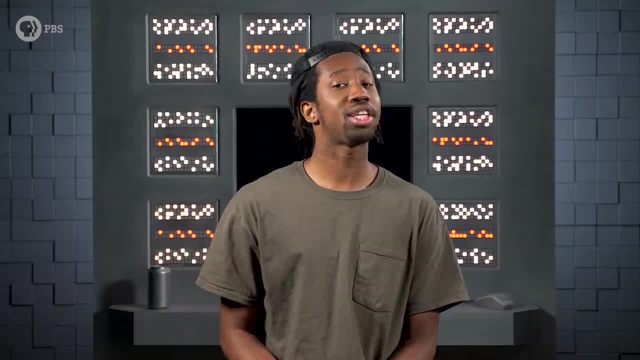 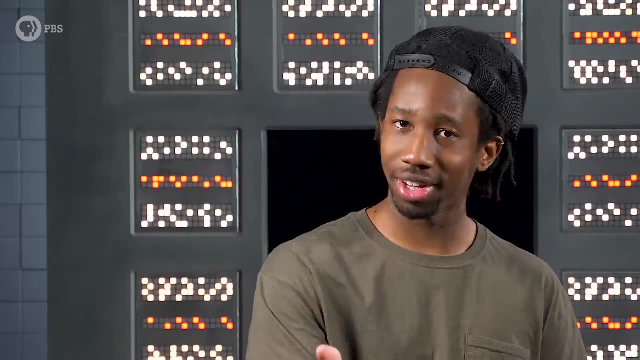 up and moving forward and then figure out what steps they took to get to that point. The longer the AI stands up and moves forward, the longer it's walking and the more rewarding it gets. So you can kind of see how the key to reinforcement learning is just trial. 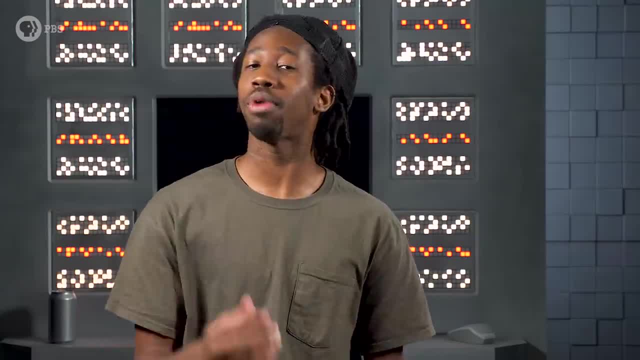 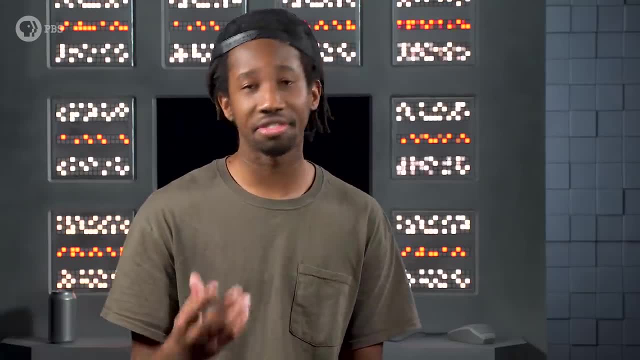 and error over and over again. For humans, a reward might be a cookie or the joy of winning your board game, But for an AI system, a reward is just a small positive signal that basically tells it: good job and do that again. 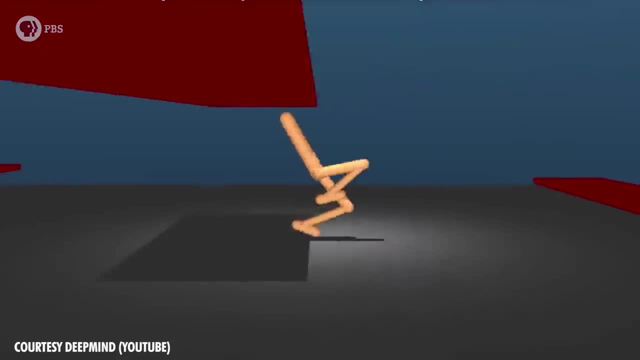 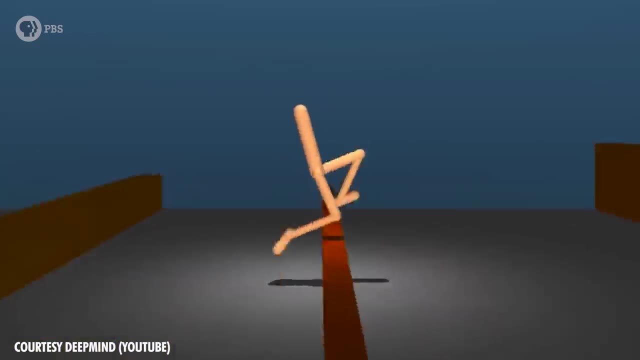 Google DeepMind got some pretty impressive results when they used reinforcement learning to teach virtual AI systems to walk, jump and even duck under obstacles. It looks kind of silly but works pretty well. Other researchers have even helped real-life robots learn to walk. 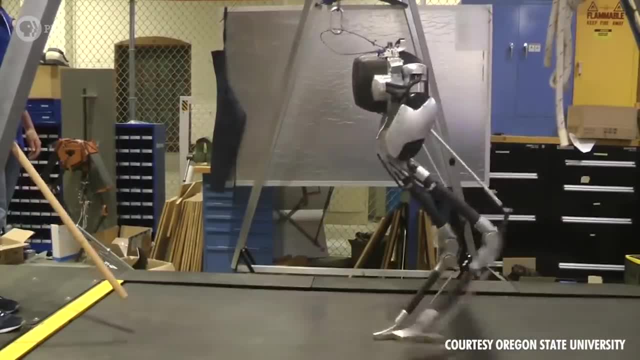 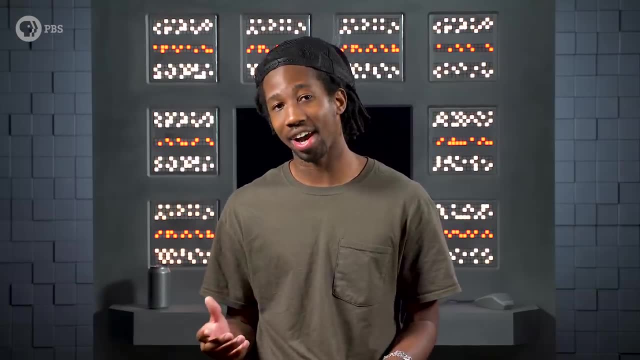 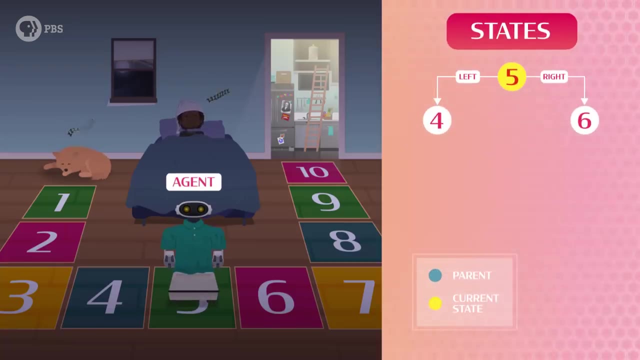 Seeing the end result is pretty fun and can help us understand the goals of reinforcement learning. But to really understand how reinforcement learning works, we have to learn new language to talk about these AI and what they're doing. Similar to previous episodes, we have an AI or agent that is our loyal subject. that's. 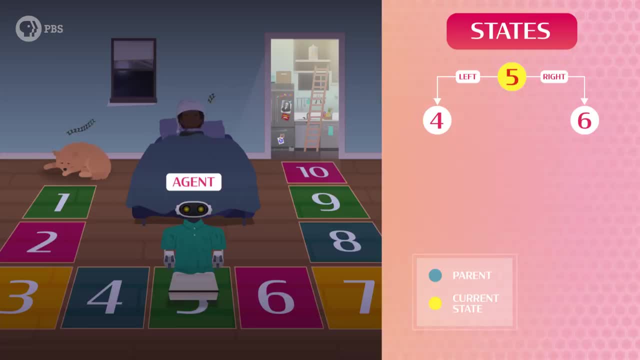 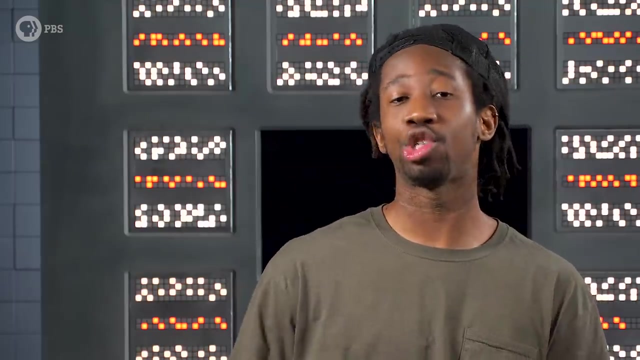 going to learn. An agent makes predictions or performs actions Like moving a tiny bit forward or picking the next best move in a game, And it performs actions based on its current inputs, which we call the state In supervised learning. after each action, we would have a training label that tells: 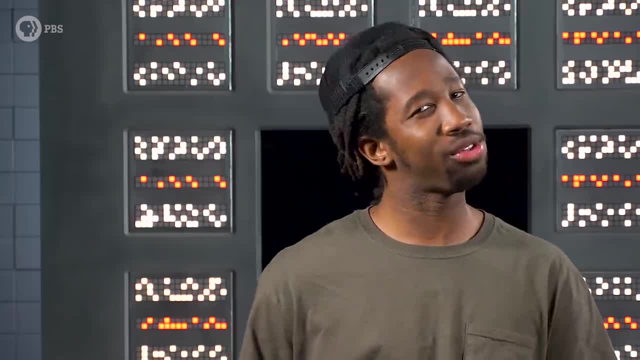 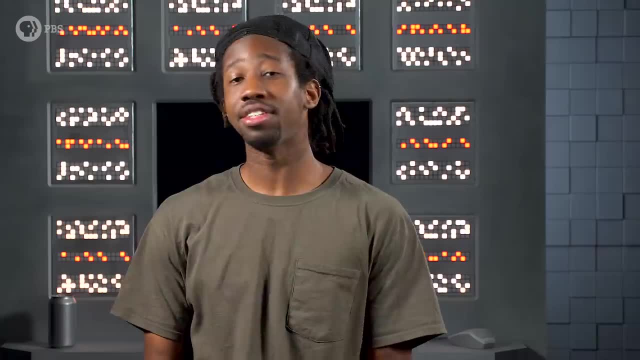 our AI whether it did the right thing or not. We can't do that with reinforcement learning, because we don't know what the right thing actually is until it's completely done with the task. This difference actually highlights one of the hardest parts of reinforcement learning. 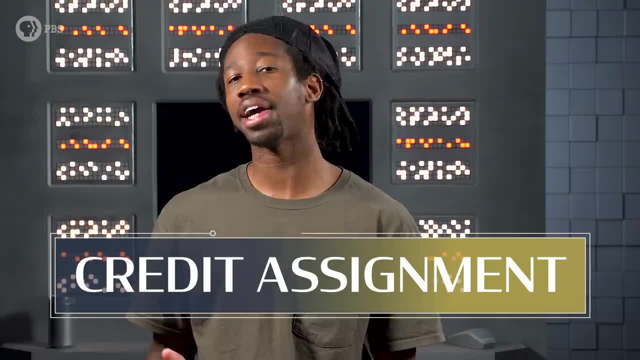 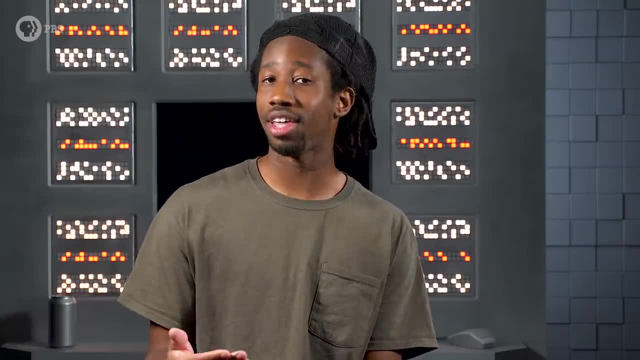 called credibility Credit assignment. It's hard to know which actions helped us get to the reward and should get the credit, And which actions slow down our AI when we don't pause to think after every action. So the agent ends up interacting with its environment for a while, whether that's 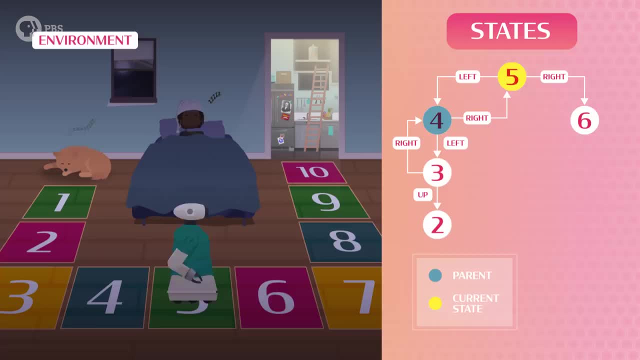 a game board, a virtual maze or a real-life kitchen And the agent takes many actions until it gets a reward which we give out when it wins a game or gets that cookie jar from that really tall shelf. Then every time the agent wins. 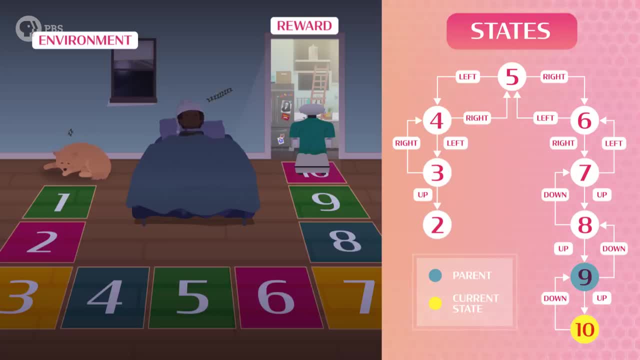 Or succeeds at its task. We look back on the actions it took and slowly figure out what game states were helpful and which ones weren't. During this reflection, we're assigning value to those different game states and deciding on a policy for which actions work best. 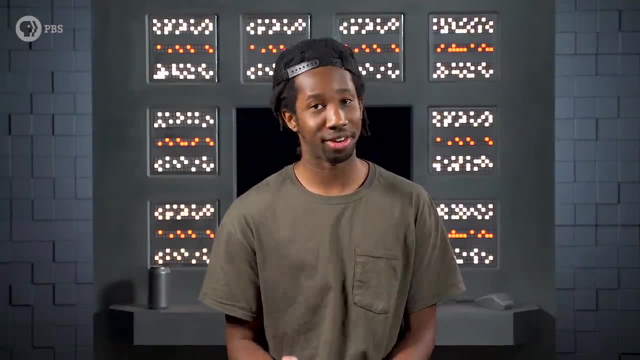 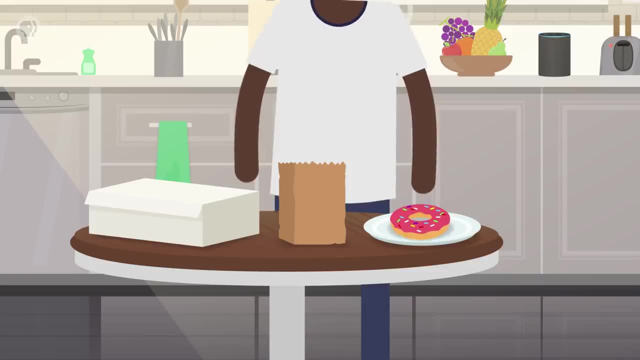 We need values and policies to get anything done in reinforcement learning. Let's say I see some food in the kitchen- A box, a small bag and a plate with a doughnut. So my brain can assign each of these a value, A numerical value. 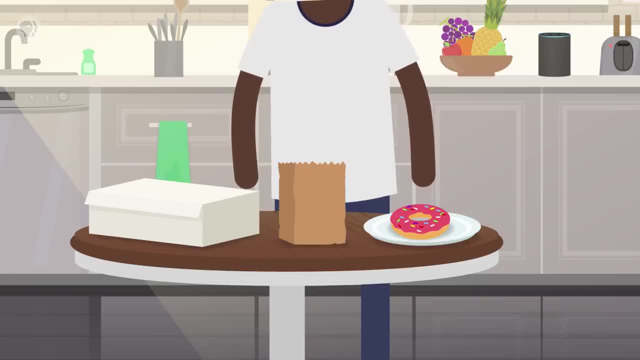 A numerical value, A numerical yumminess value. The box probably has 6 doughnuts in it, the bag probably has 2, and the plate just has 1.. So the values I assign are 6,, 2, and 1.. 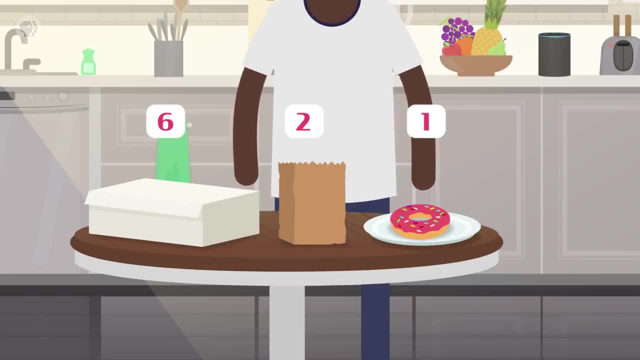 Now that I've assigned each of them a value, I can decide on a policy. to plan what action to take, The simplest policy is just to go to the highest value. that box of possibly 6 doughnuts, But I can't see inside of it and it could be a box of bagels, so it's high risk, high. 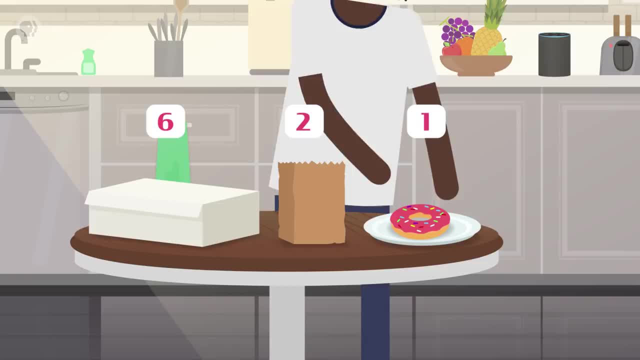 reward. It could be low reward, but low risk, Going with the plate with one guaranteed delicious doughnut. Personally, though, I'd pick a middle-grown policy and go for the bag, because I have a better chance of guessing that there are doughnuts inside a bag than the box. 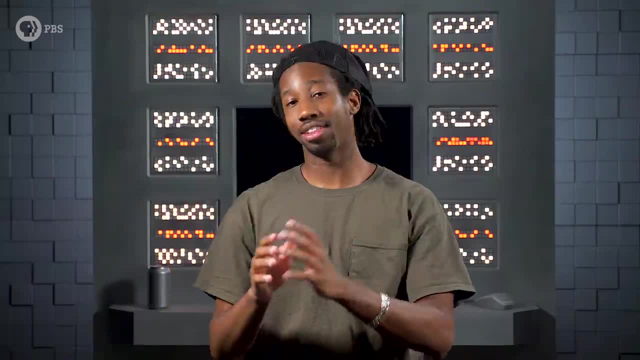 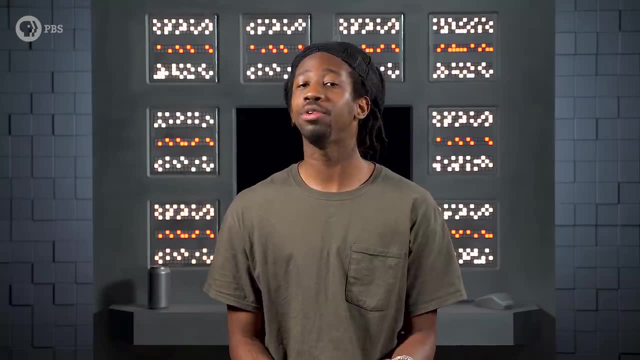 And a value of one doughnut just isn't enough. That's a lot of vocab. so let's see these concepts in action. Our example is going to focus on a mathematical framework that can be used with different underlying machine learning techniques. Let's say John Greenbot wants to go to the middle ground. 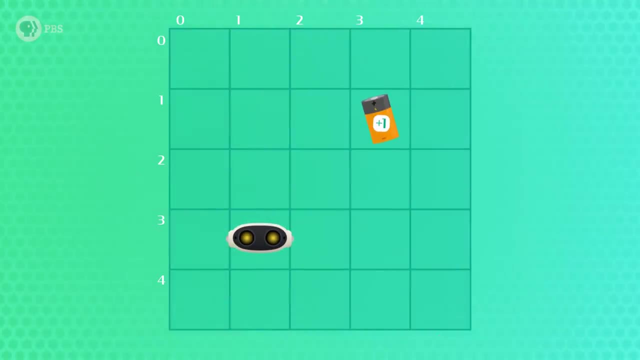 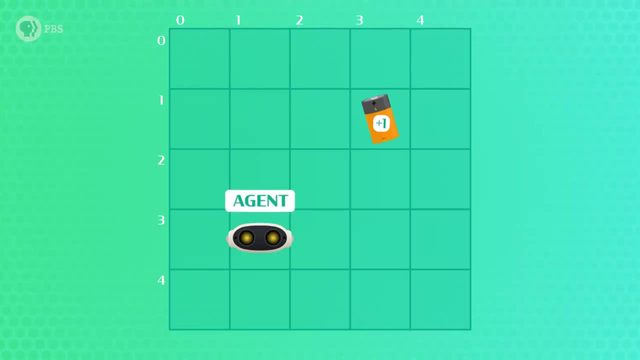 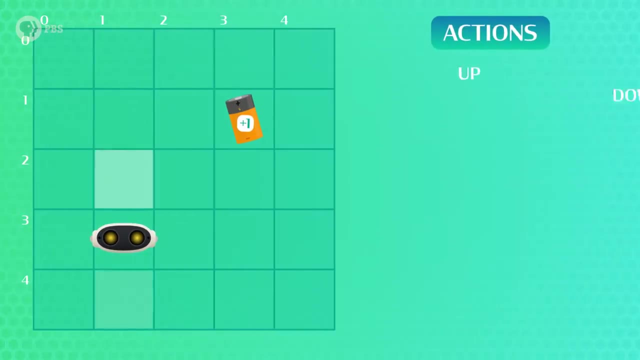 In this example, John Greenbot is a brand new agent and the room is the environment he needs to learn about. From where he is now in the room, he has 4 possible actions: Move up, down, left or right, And his state is a couple of different inputs. 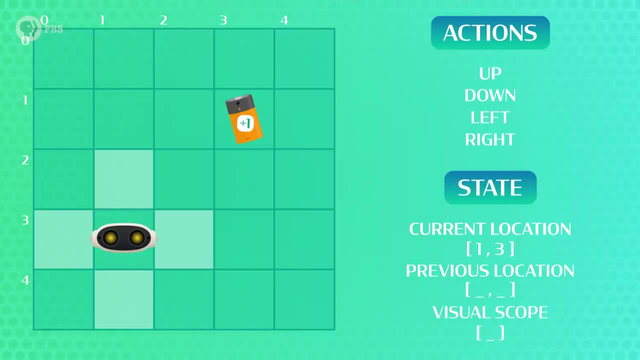 Where he is, where he came from and what he sees. For this example, we'll assume John Greenbot can see the whole room. So when he moves up or any direction, his state changes, changes, But he doesn't yet know if moving up was a good idea because he hasn't reached the 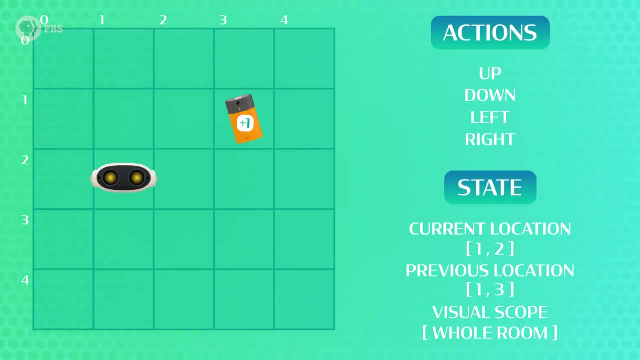 goal. So go on. John Green, Bot explore. He found the battery. So he got a reward, that little plus one. Now we can look back at the path he took and give all the cells he walked through a value, specifically a higher value for those near the goal and a lower for those further away. 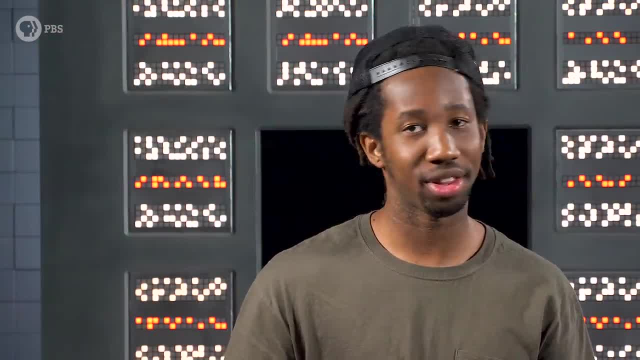 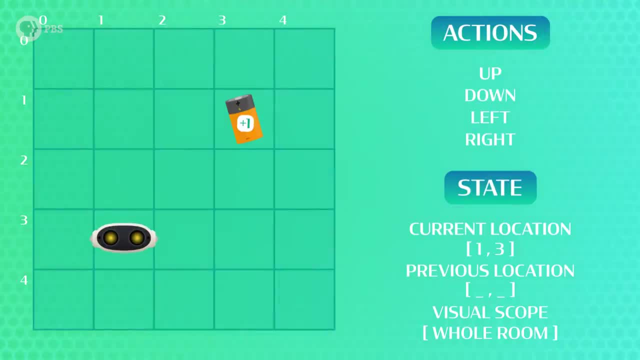 These higher and lower values help with the trial and error of reinforcement learning, and they give our agent more information about better actions to take when he tries again. So if we put John Green Bot back at the start, he'll want to decide on a policy that maximizes. 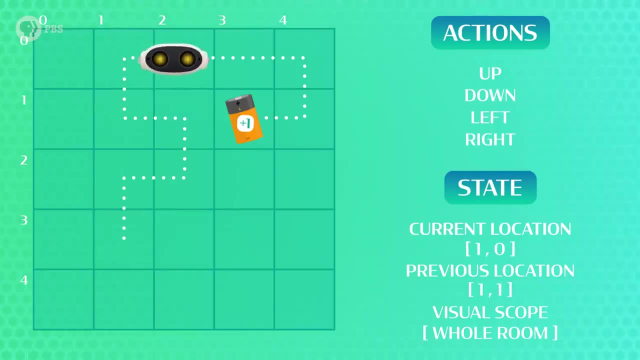 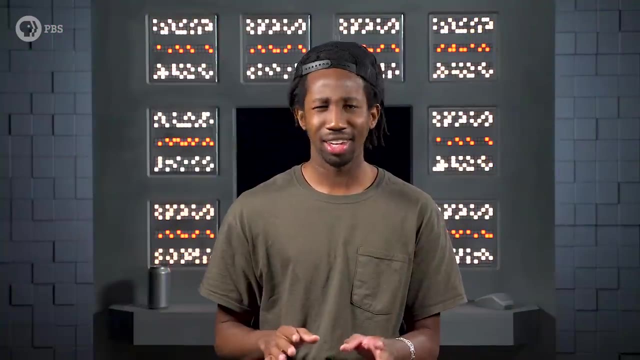 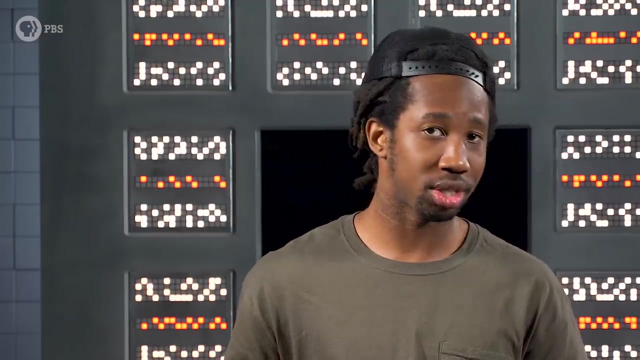 reward. Since he already knows a path to the battery, he'll walk along that path and he's guaranteed another plus one. But that's too easy And kind of boring if John Green Bot just takes the same long winding path every time. So another important concept in reinforcement learning is the tradeoff between exploitation. 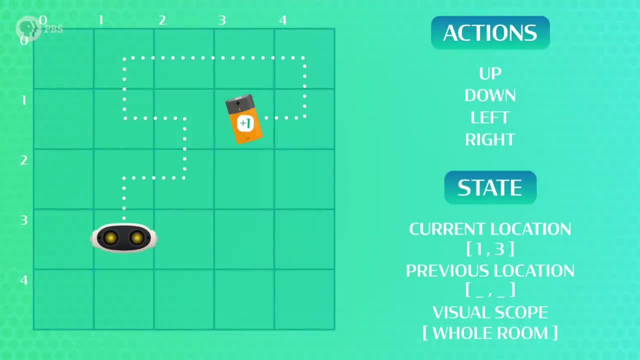 and exploration. Now that John Green Bot knows one way to get the battery, he could just exploit his knowledge by always taking the same ten actions. It's not a terrible idea. He knows he won't get lost and he'll definitely get a reward. 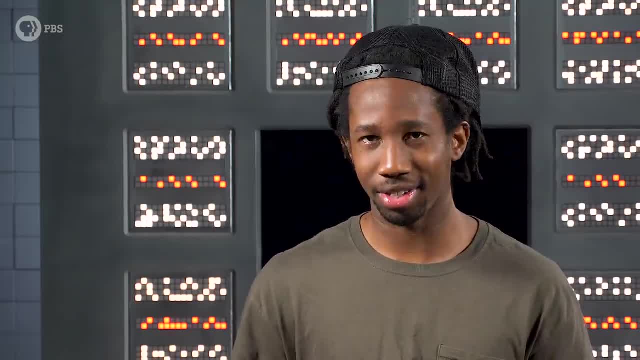 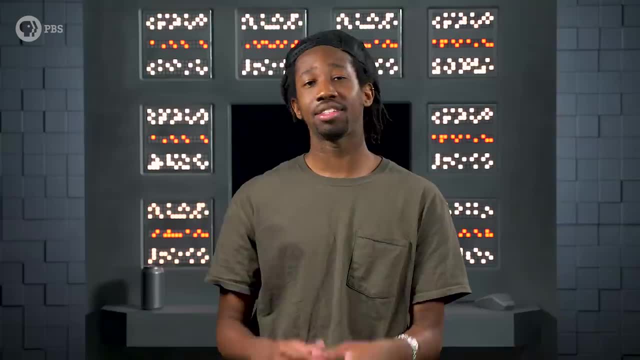 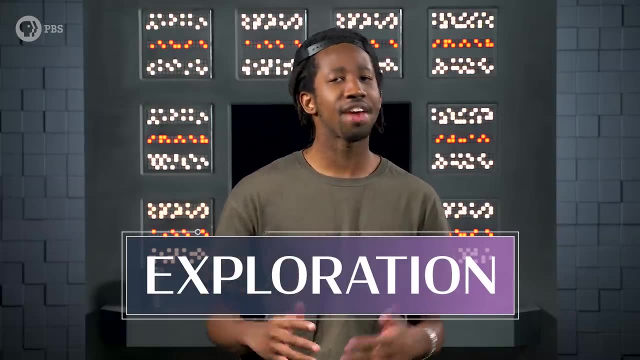 But this ten action path is also pretty inefficient. There are probably more efficient paths out there, so exploitation may not be the best strategy. It's usually worth trying lots of different actions to see what happens, which is a strategy called exploration. Every new path that John Green Bot takes will give him a bit more data about the best ways. 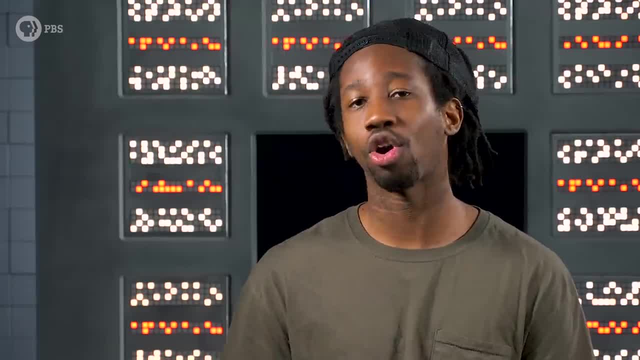 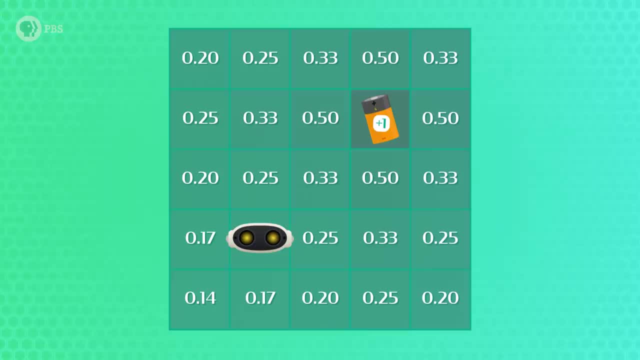 to get a reward. So let's let John Green Bot explore for 100 actions, and after he completes a path, we'll update the values of the cells he's been to. Now we can look at these new values. During exploration, John Green Bot found a shortcut, so he knows a path that only takes. 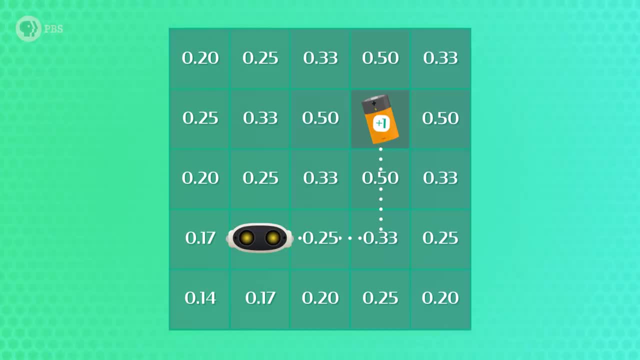 4 actions to get to the goal. This means our new policy, which always chooses the best value for the next action, will take John Green Bot down this faster path to the target. That's much better than before, but we paid a cost. 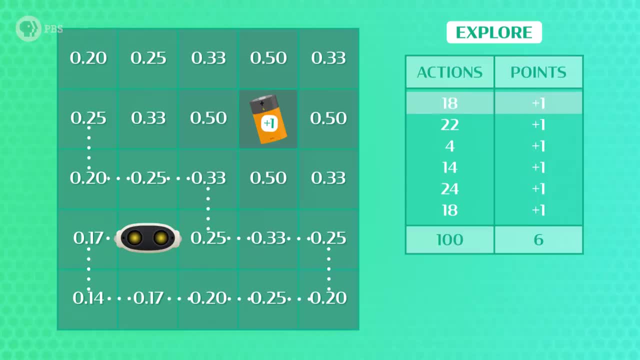 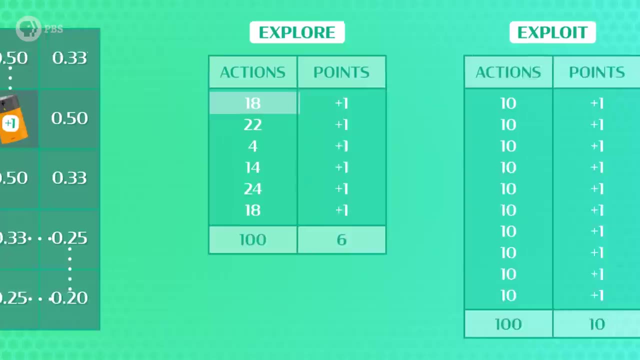 Because during those 100 actions of exploration he took some paths that were even more inefficient than the first ten action path and only got a total of 6 points. If John Green Bot had just exploited his knowledge of that first path for those 100 actions. 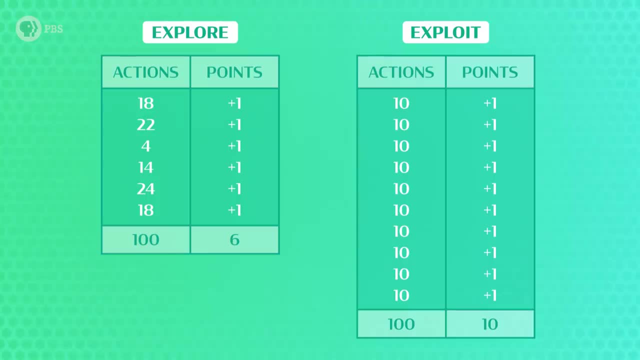 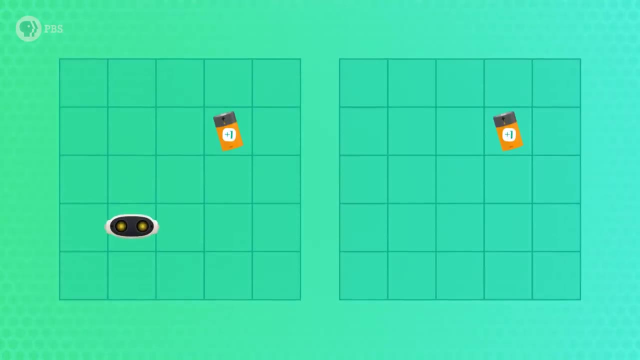 he could have made it to the battery 10 times and gotten 10 points. So you could say the exploration was a waste of time. But if we start a new competition between the new John Green Bot, who knows a 4 action path, and his younger, more foolish self, who knows a 10 action path, over 100 actions, the 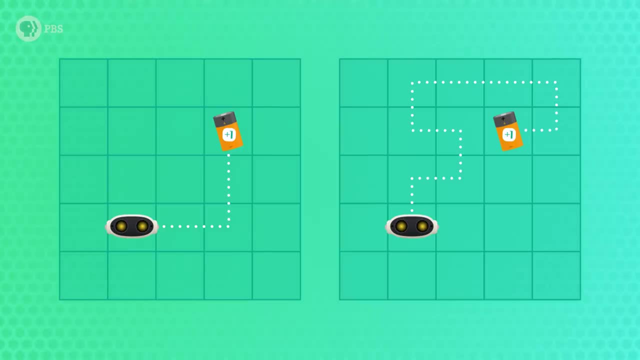 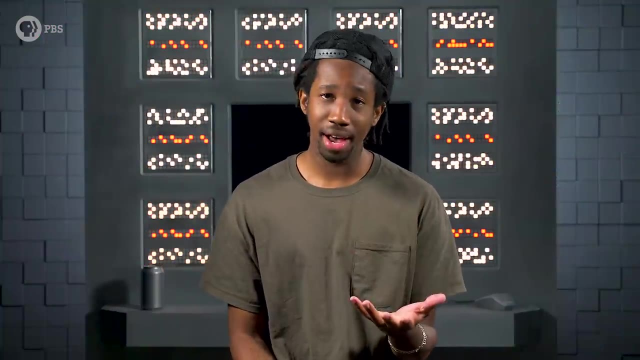 new John Green Bot will be able to get 25 points because his path is much faster. His reinforcement learning helped. So should we explore more to try and find an even better path, Or should we just use exploitation right away to collect more points? 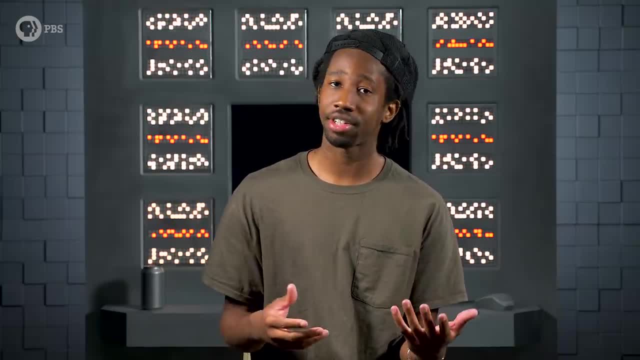 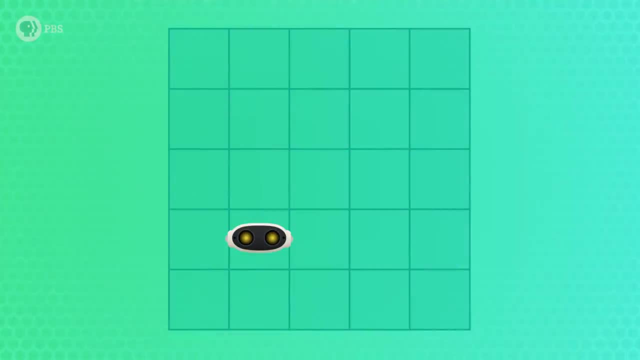 In many reinforcement learning problems. we need a balance of exploration and exploitation, and people are actively researching this tradeoff. These kinds of problems can get even more complicated if we add different rewards, like a plus 1 battery and a plus 3 bigger battery. 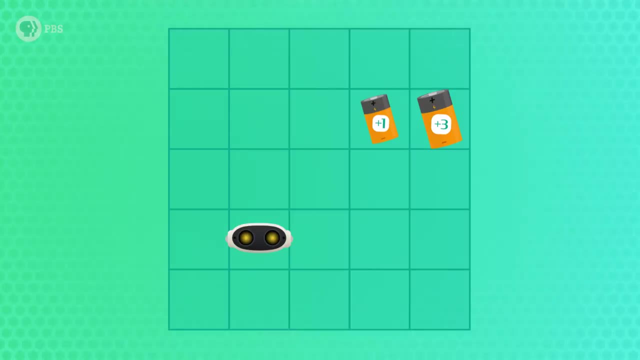 Or there could even be negative rewards that John Green Bot needs to learn to avoid, like this black hole. If we let John Green Bot explore this new environment using reinforcement learning, sometimes he falls into the black hole. So the cells will end up having different values than the earlier environment and there 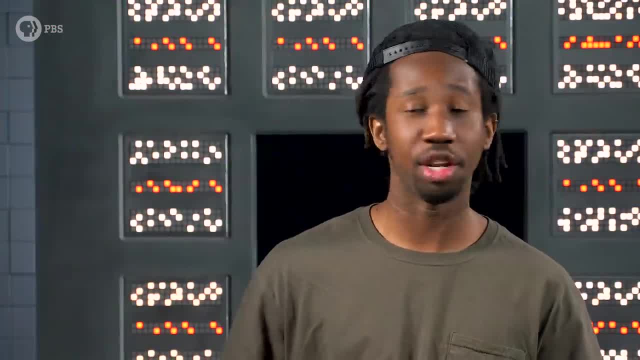 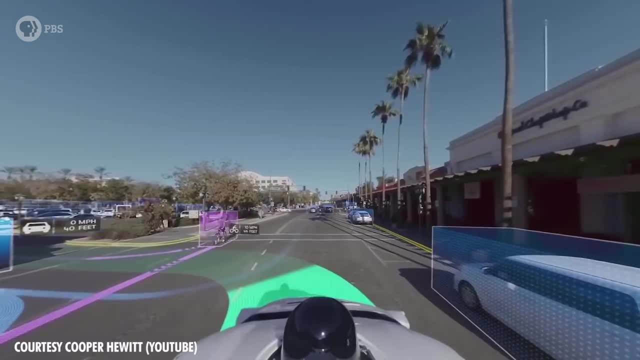 could be a different, best policy. Plus, the whole environment can change in many of these problems. If we have an AI in our car helping us drive home, the same road will have different people, bicycles, cars and black holes on it every day. 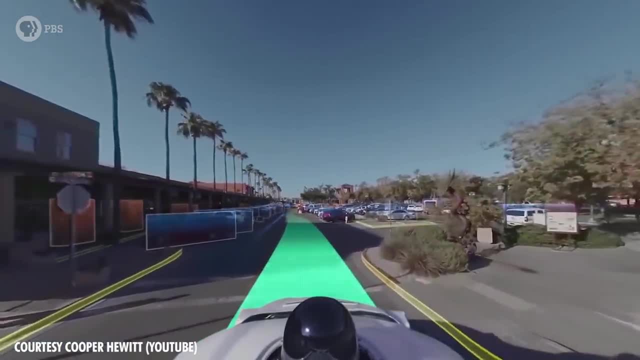 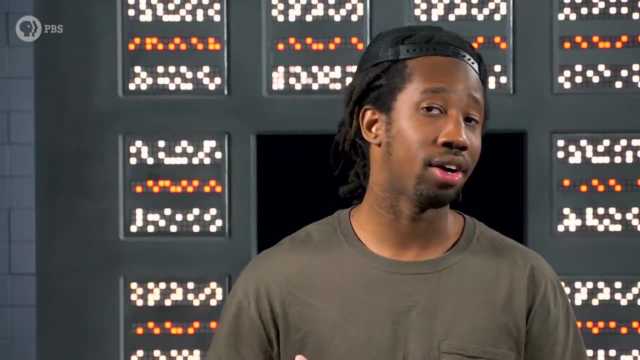 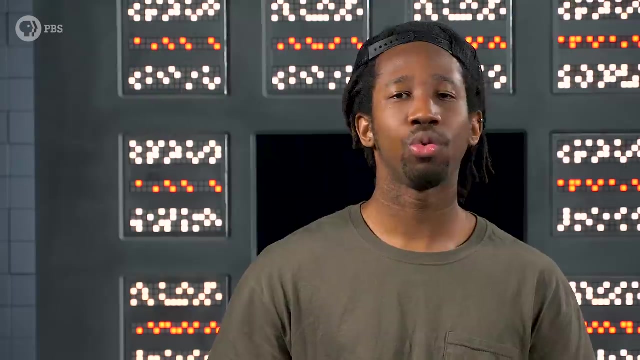 There might even be construction that completely reroutes us. This is where reinforcement learning can be a big help. When John Green Bot was learning how to navigate on that small grid, cells closer to the battery had higher values than those further away, But for many problems we want to use a value function to think about what we've done. 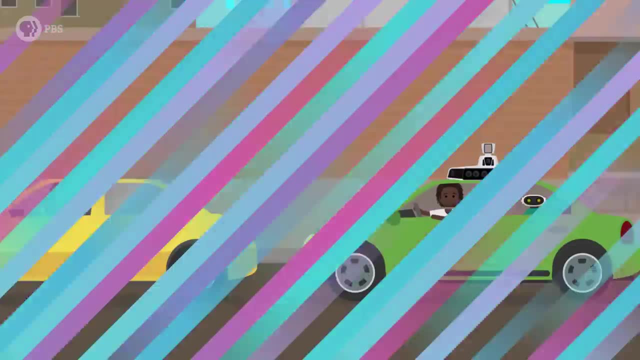 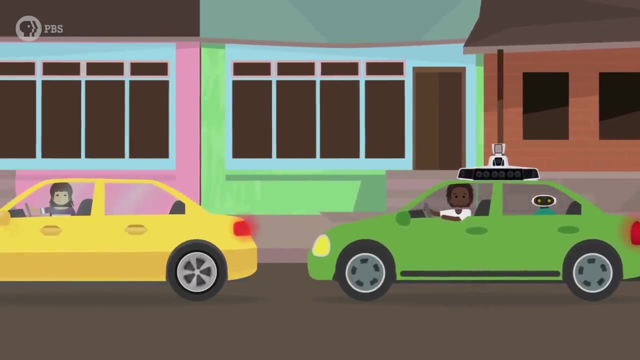 so far and decide on the next move, using math, For example, in this situation where an AI is helping us drive home. if we're optimizing safety and we see the brake lights of the car in front of us, it's probably time to. 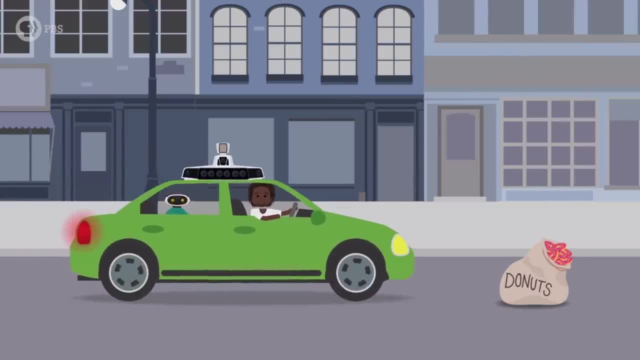 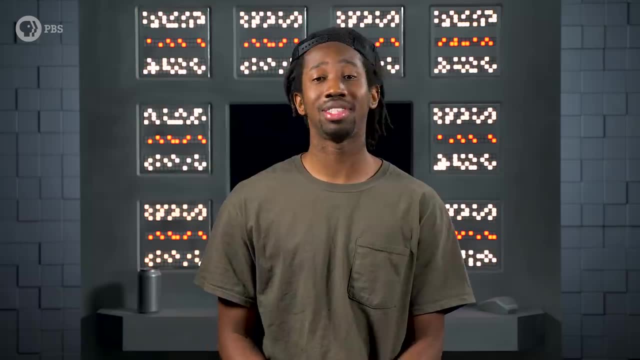 slow down, But if we saw donuts in the street we want to stop. So reinforcement learning is a powerful tool that's been around for decades, But a lot of these problems need a ton of data and a ton of time to solve. 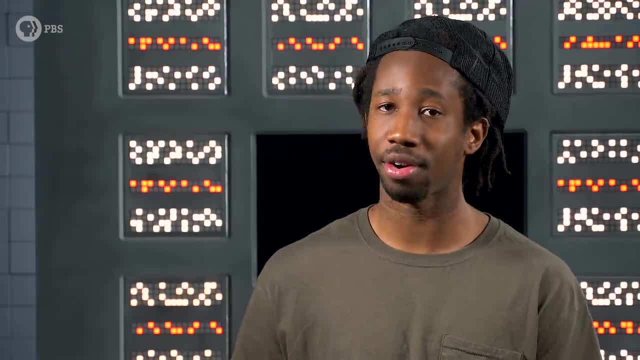 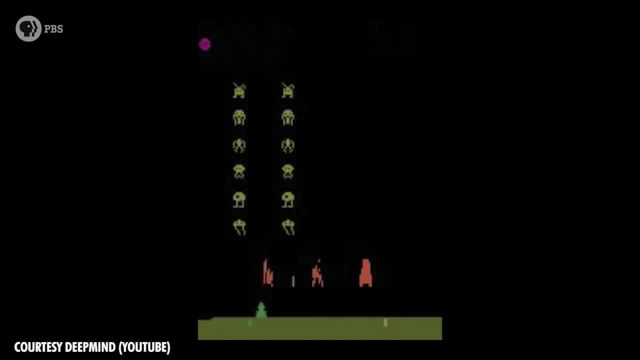 There have been really impressive results recently thanks to deep reinforcement learning on large-scale computing. These systems can explore massive environments in a huge number of states, leading to results like AIs learning to play games. At the core of a lot of these problems are discrete symbols.